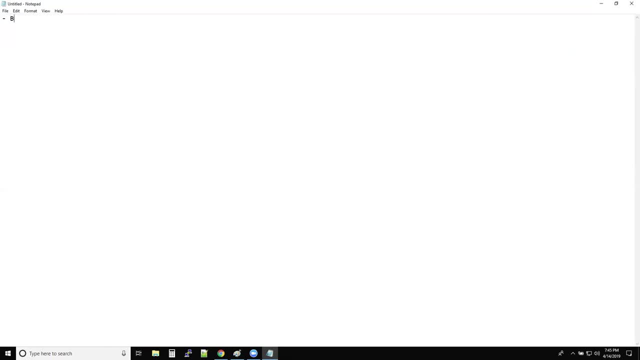 I can prove you this point. Let me write it: Business logic. Sometimes it's a problem with the business logic. I'll give you one example. Let's take you go to bank and there is one teller and there is one manager. All right, So every day, whenever, okay, whenever people are coming to the teller and asking: 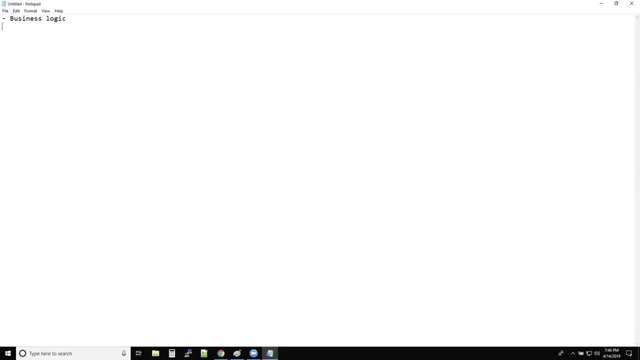 the teller to give them $100, the detailer is a teller is authorized to approve the bills or the request till $100.. For any request that is above $100, the customer has to wait to meet to the manager. Right Now, this is a general scenario, where there is one teller and there is one manager. So as for the business logic we see, 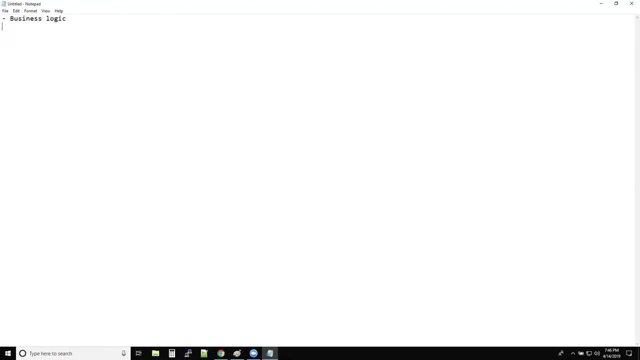 that generally people like out of 100, only one person or two person will go for withdrawing money above $100. That is like when the bank started. Now, after some time, what happened? because the economy grows and people are getting handsome salaries, or people got great appraisal or hike at their office- they start withdrawing more money. Now, in that case, what happens is: 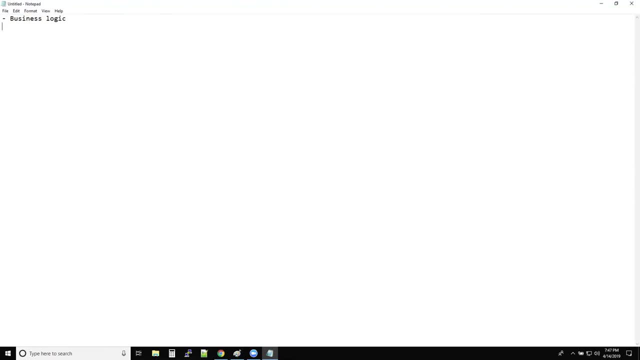 like out of 100, 60 people generally tend to withdraw more than $100 in one transaction. So at any given point of time in the bank there were 60 people out of 100, they are 60% of the people. they are always waiting for the manager to approve their transaction. Now this causes the waiting. this is a business logic problem. So how can you solve this problem? 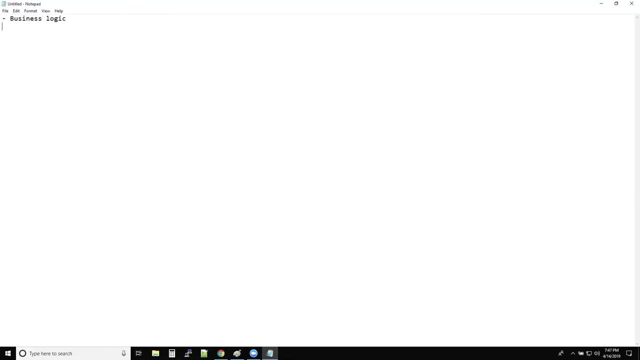 So what bank can do is they can allow the teller saying like: Hey, we will increase your authority to release any amount that user is requesting that is below $500. So that way what will happen is people will not wait for the manager until they're withdrawing above $500. A simple example, but the same can be applied in business world or your application team. 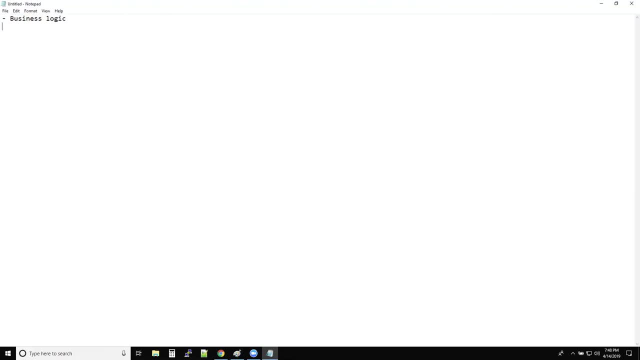 Or it depends like where exactly the problem is. what rule in the business if we change, that might completely avoid the problem that might happen Like. one simple example that we saw just now was if can we reschedule the admin backups to a different time, because exactly at the same time there is something else going on And guys forget about admin backups. I'll give you a real world scenario. 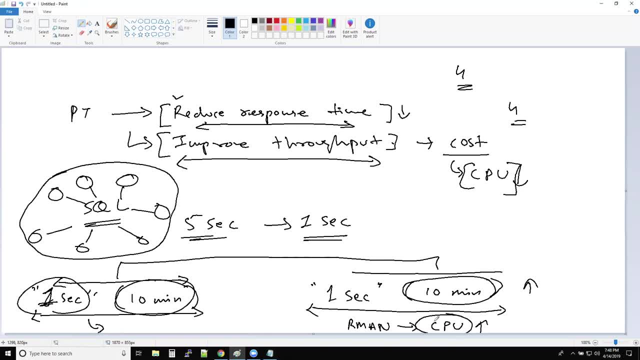 On the servers where you host your databases, there is always OS level team that is working, there is always storage team that is working and there is also network team that is working. So it's not always that things that belong to DBA that causes CPU impact. there might be a network activity that is going on on the server that is causing high CPU utilization And because of that application, there might be a network activity that is going on on the server that is causing high CPU utilization. 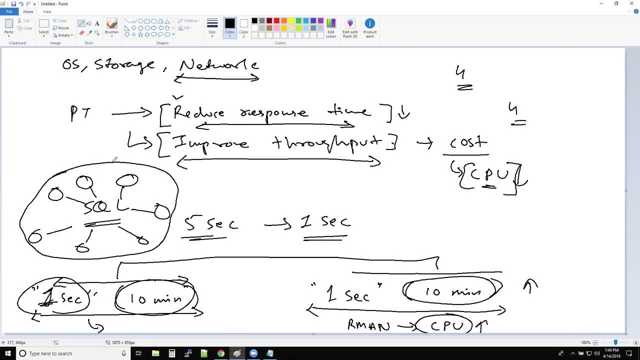 The CPU usage is very high. Ultimately it causes or impacts your database. The same goes with the storage team, same goes with your operating system team. So don't always be ready to take the blame, Like don't always say that because of the database things are running slow. No, because of other teams also things might run slow. So let's come back to the steps. The step number one is in performance tuning. can we change the? 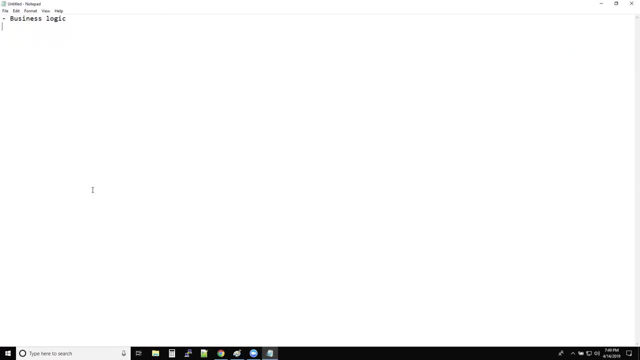 business logic in a way that completely avoids the problem, And this happens only when you work with your client, work with your application team. So the best way to have great business logics is that at the time of the development of the application, or when people are developing, it is good to have everyone in that meeting. Most of the times, what happens is the front end team and the back end team, like the. 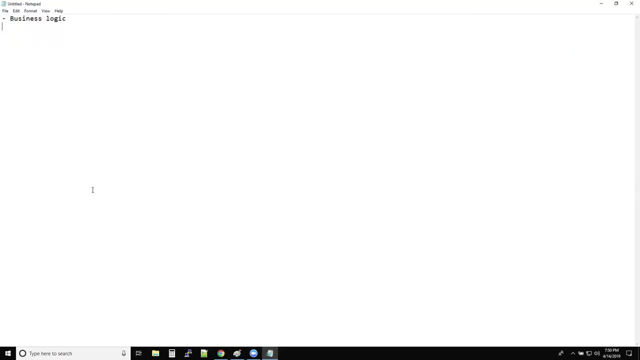 developers and database architect. they will sit and design the application. So in the same meeting it is always good to have a network architect guy, it will. it is always good to have a storage architect guy. And when they sit and design the applications, definitely they, their recommendations, are more important. So business logic is very good If you define it even before the application is built, because once the application is built, based on a 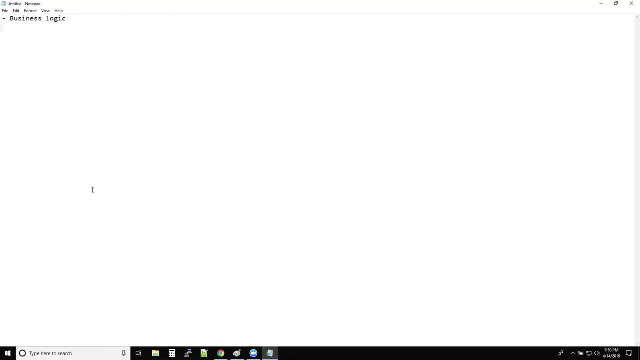 logic, It's always hard to go back and, kind of like, make changes to the application. So the first things first is the business logic, how business logics are defined And, like the bank example, a simple business change allowing the teller to increase. 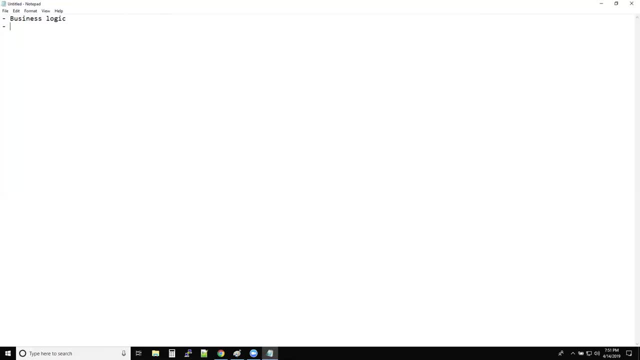 their capability to release any amount that is below $500 will change. the game are. and then those 60% of切, the people who are waiting. That's nothing but queries that are waiting inside the database, right? So if we can change that, 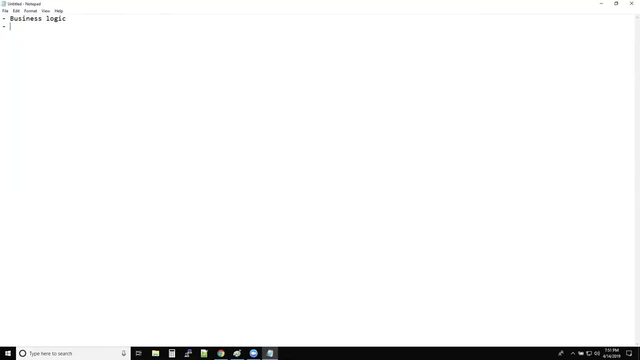 logic, then the number of people waiting will change. The second step, of course, business logic. it can only be done, or it is always good, to work on business logic when application is being developed. The second one is changing or designing the data. 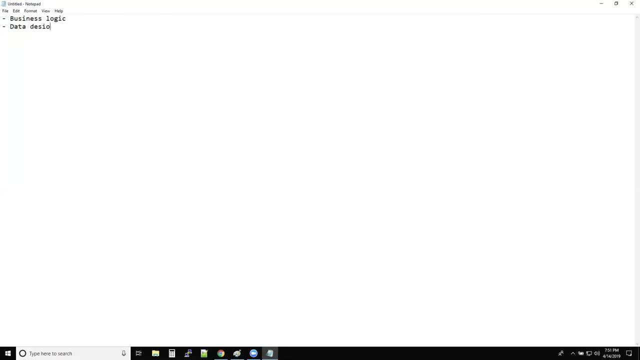 and okay, let me write it: data design. This data design, the most important part in the data design is the database normalization And I think in the skill sessions- if some students who are part of my SQL training- we have done and done. 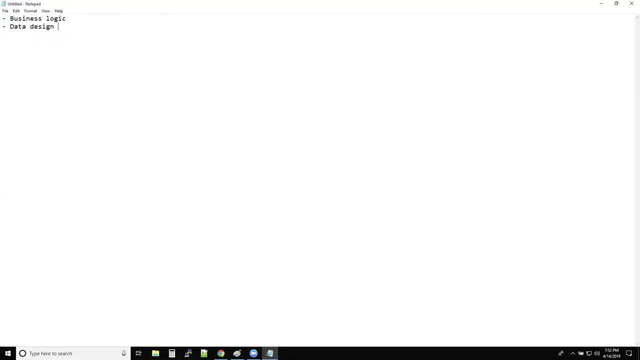 a little bit of database normalization, moving the data from first normal form to second normal form and then third normal form. So the data design, the phase when, when the database developer is sitting with the client and designing the tables inside the database. that is very important. So how well the data is normalized is. 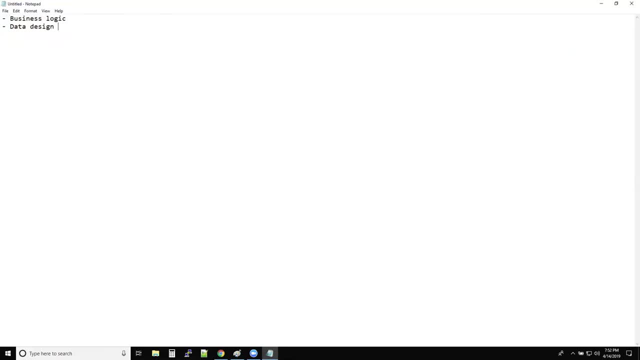 something also impacts your database performance. So it's not always like the query, it's not always the indexes, it's not always statistics. there are more things to a performance issue. So the first one is business logic. Second is data design. that's nothing but the. 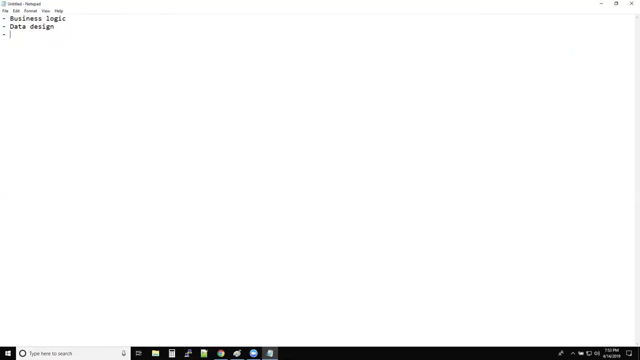 normalization. The third one should be the logical structures inside the database, But no, I think before the logical structures. now that data design is going on, the application design. application design is also very important: How well the code is written. Can we make changes to the code in? 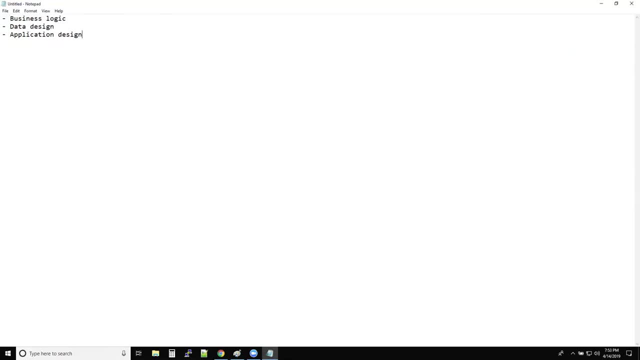 a way that will avoid deadlocks, Like a simple example that we just now see? can we make some changes to our application that will reduce the wait time for a session so that a lock is not acquired before the query is executed? Can we make an update? 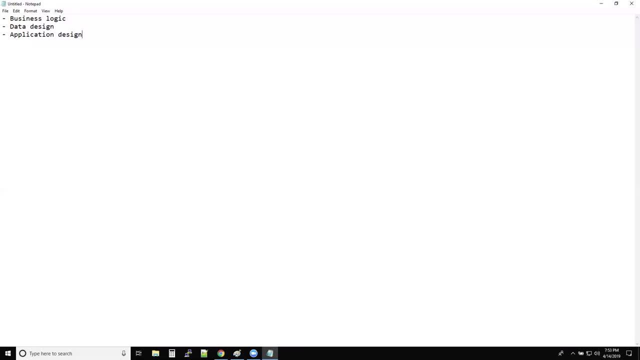 to our application code. that will make sure that all the code will run smoothly, evenly throughout 24 hours. Can we distribute the code like that? Can we make sure? can we schedule the database tasks in a different way that do not collide with the arm and backups? if they're running Can, can we? 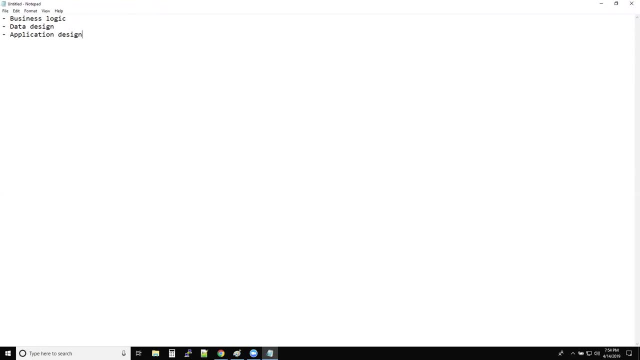 schedule or ask the OS level team to run their application at a different time so that it does not collide with the arm and backup schedule. So there are a lot of stuff that happened inside the database So. but as a DBA you will deal with the database and 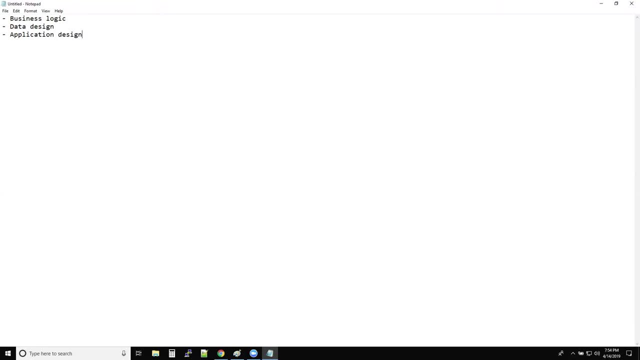 application right. So the application design is more important, how well the code is written, how well the SQL queries are written, how well the queries avoid the locks or deadlocks, how well the queries do not kind of like bother each other. right, So the application code is more important. at the 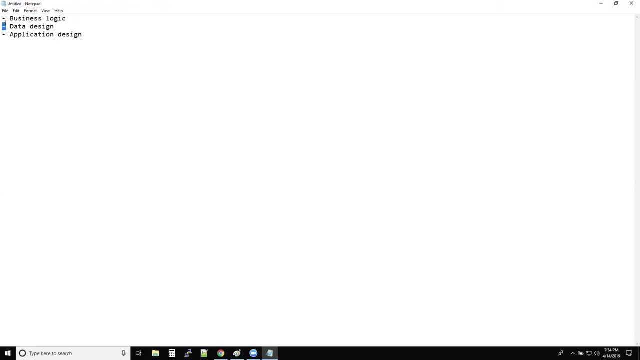 stage. So first is business logic. can we change a business logic that completely removes the problem? Can we renormalize the data Or is there a requirement to normalize the data again inside the database that might change the performance of the database? Is there a change in the application code that? 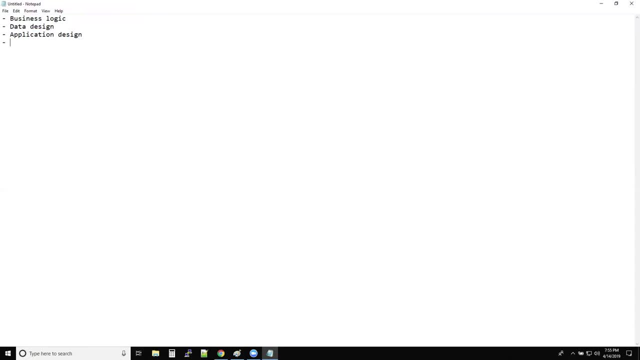 will avoid a deadlock, So we'll use the deadlock example over here. Now we can assume. now can you believe these all are external stuff? This is not yet inside the database, right? This is like you're working on business logic, you're working on the data design and you're. 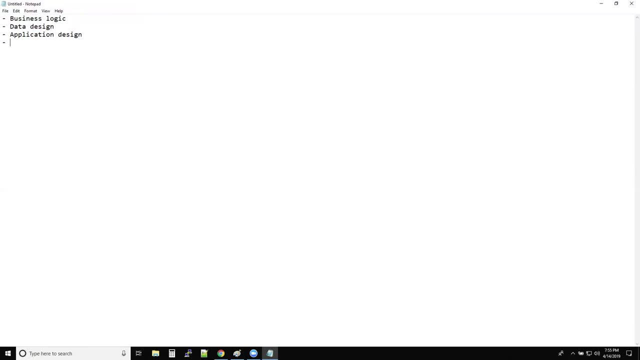 working on the application design. Till now we haven't entered inside the database, right. So these three are the primary prime. sorry, the primary performance tuning steps are all outside the database. This is very important details, guys. Now that, okay, you're done with. 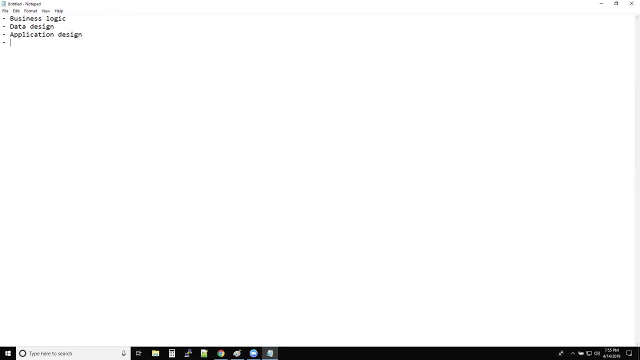 everything outside the database. Now, slowly you get inside the database and you see can we make changes to the structure of the database, Change database structure. Now, when we talk about the database structure, of course can we introduce indexes inside the table. that will improve the readability of. 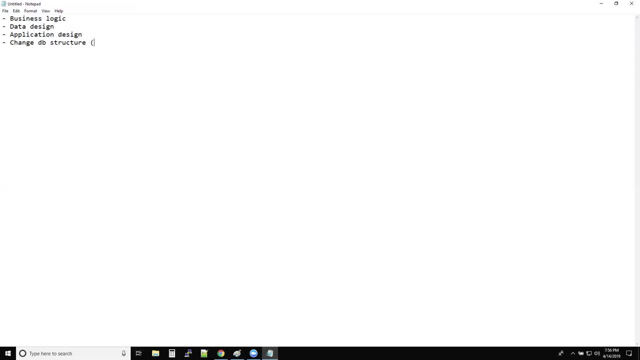 the data. And guys, don't worry, I'll take some time in today's session to talk about indexes, because even that is more important for when it comes to performance tuning right. So indexes, Can we introduce indexes inside the database? that will improve the database. 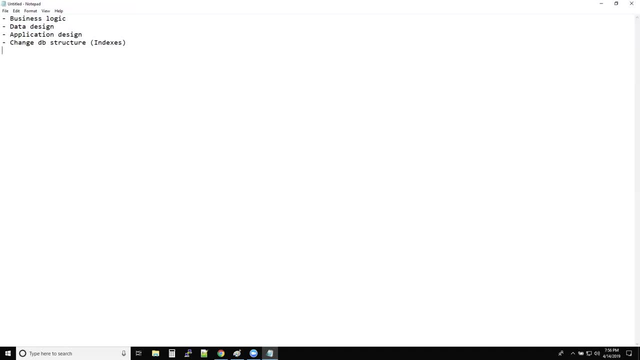 or the query performance, And you won't believe exactly at this stage. once you're done with these steps, then you technically get into the tuning of the SQL. tuning the SQL, can we efficiently change the SQL query in order to make sure it is running perfectly fine? I'll give you a quick examples. 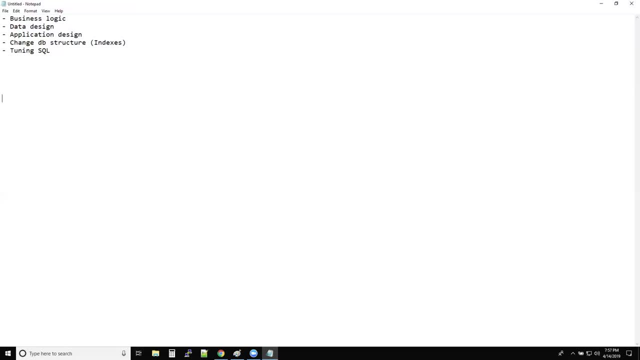 couple of examples that might help you guys to understand what I'm talking about. So let me pull up the paint and then we'll come back to this one. So what do you mean by effective SQL? assume that there is a table and there is a column called. 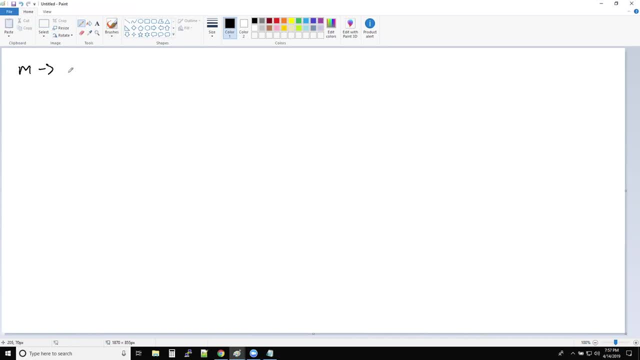 as gender And we know that we have 80% male and then we have 20% female records inside the database. I'm just creating a scenario, guys. Now, in this kind of situation, let's take you are saying: select all the records from the table where 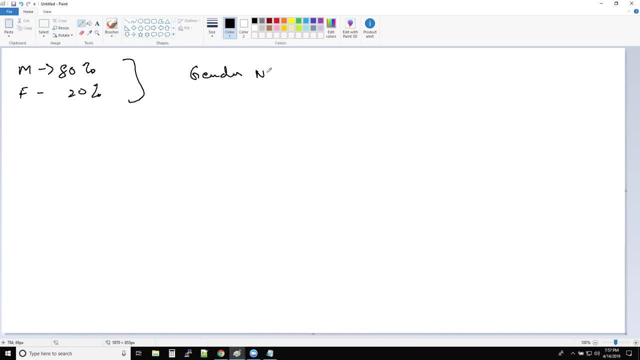 gender is not equal to male. So what you are doing over here, you are actually telling the query first compare if gender is equal to male and then you are negating it. That means you are pushing 80% of the records inside the query. All right, this is a simple example. So, rather, 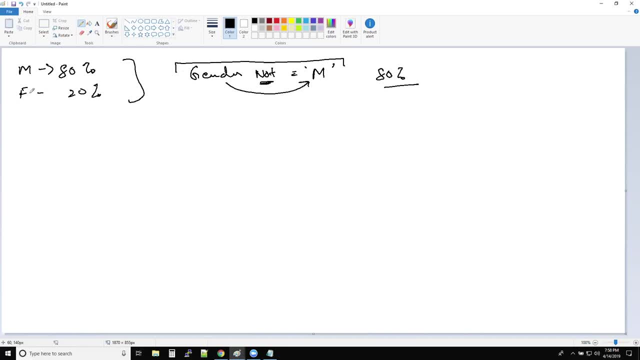 than this. if you can check the data inside the query- Sorry, your gender column- and you see there are only two possible values, like male and female, then can we rewrite the statement saying like: gender is equal to female. right now, if you see this one, you are. 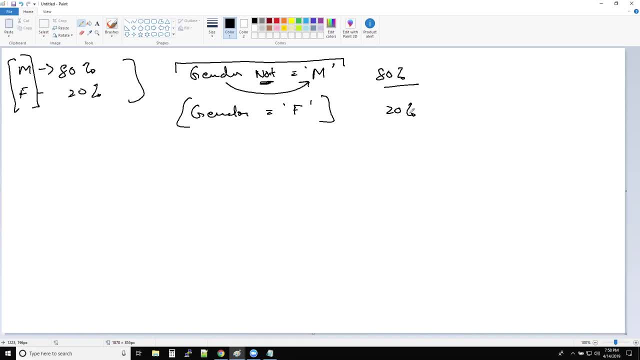 pushing like 20% records inside the SQL again, guys. I'll give you one more example. if you are joining tables- okay, let's take you are joining table one- you're joining table one on table two and table two on table three. in this one, guys, in your join condition the table one like the where. 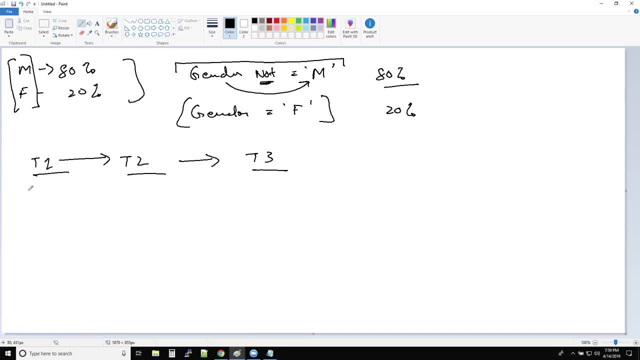 clause: when you are joining, the table one is returning 1000 records, table two is returning two records and then table three is returning maybe 100 records. all right now, in this case, if you see your driving table or the main table inside, your join query is pushing one 1000 records. this is kind of like poor SQL. so what you can do. 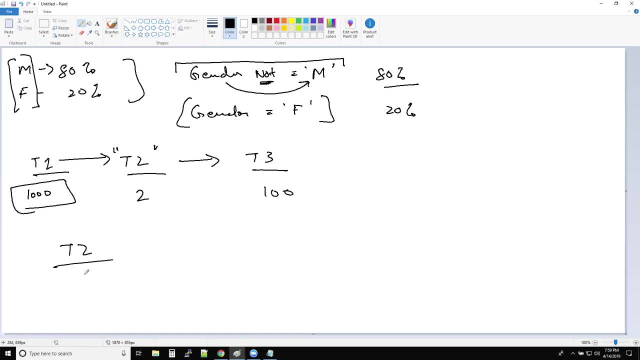 is rather you make your t2 as the driving table because this will push in only two records inside the table. technically, if it is mapped to t1, if there are two records- and let's take there are dependent records- for each two records. there are four dependent records. that means from the t1 eight records will be selected. 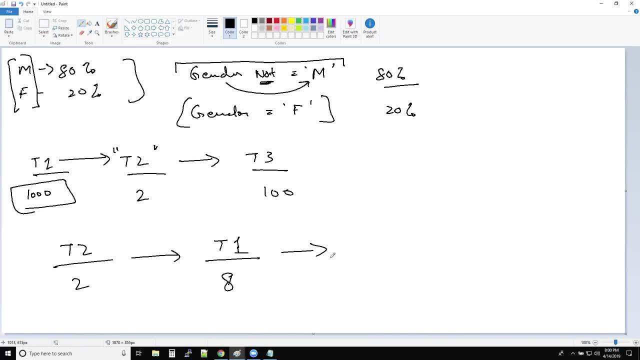 and based on t1 from t3. we are just assuming we'll keep it hundred. now do you see how the driving table or the main table inside a join query can change the complete game? so it's always like the whole thing. so everything is over and done. so it's always running every single. 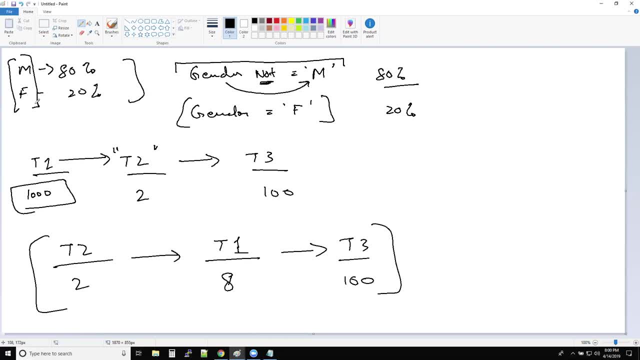 time when you're working on diets aligning, so it's always like when you walk on SQL tuning. of course, you will need to have a sense of the type of data that is going in, like, for example, for the gender example. this is one of the best examples, like you can see what type of data is and how well veía. 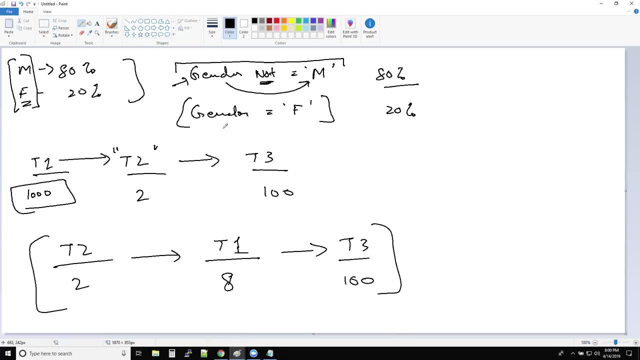 skill is written, and if it is joint statement, then definitely you see like which one is the driving table, and then can we use a table or a condition that gives us like a chodzi Jo, yup, then such data. does we are able to do this thing? not, we probably cannot, while things are fine. 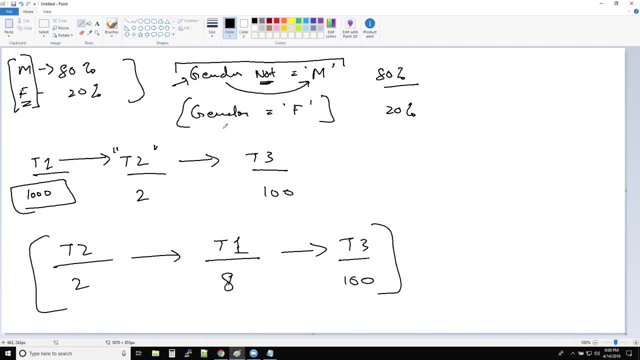 so please, for example, in case we have bad function or we're managing something, we can form a second intervention, that is, reducing the number of rows that you are pushing inside the query. So, guys, all this comes through experience. It's not one day, two day and, like you, just learn through it. It's. 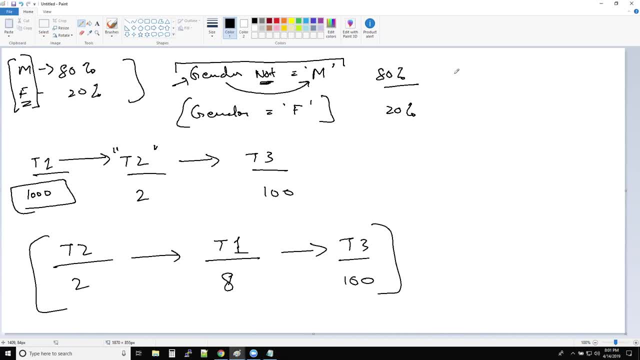 all experience, But my ultimate goal when I talk about the SQL tuning is reduce the number of records in the first instance as soon as possible. Do not allow your query to get more records and then sort: no, try to make sure your queries are selecting. 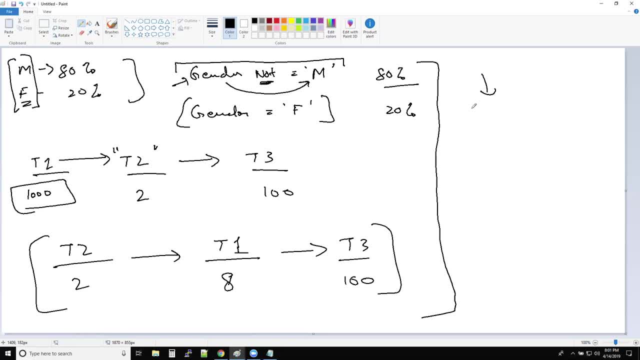 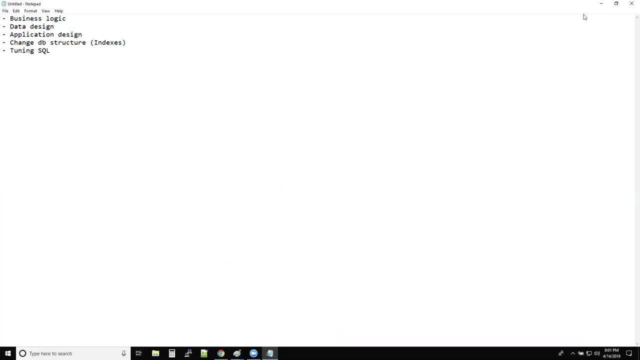 as little records as possible And kind of like. of course, there are a couple more examples that I want to give, but it will not make sense right now. So all in all, like in this case, make sure you are using a method that is pushing in. 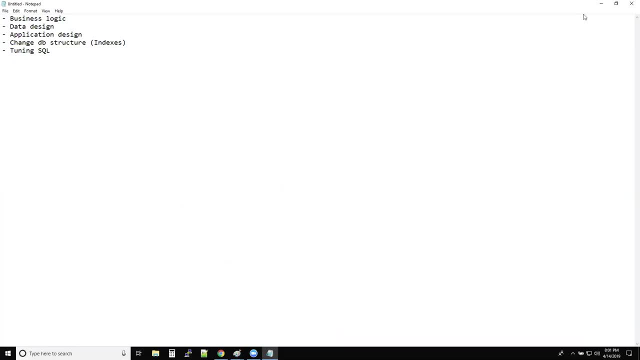 less records. So tuning of SQL is not like one task. First thing first is, if you are tuning the SQL, make sure you're always driving in less number of records as much as possible. So the goal of SQL tuning is to write effective SQLs that reduce. 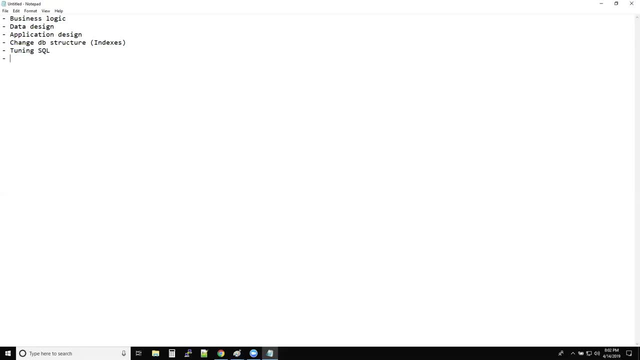 the number of records that go through your queries, right. The next one should be, of course, now that you're tuning. tuning of the SQL has to do with the number of records. That is one part. There are again other parts. The next one would be: 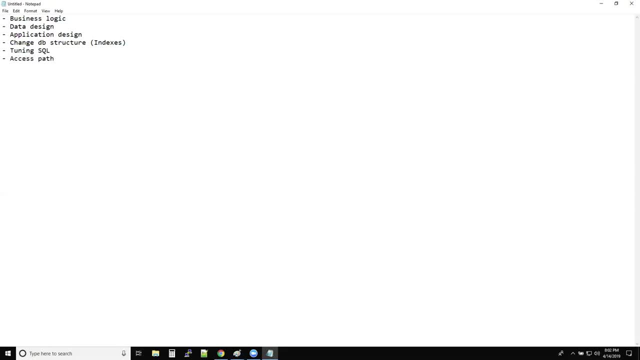 access path. This is very important And very few people get this access path. I think if there are developers, they they are pretty good with access path. But let me talk about the access path a little bit, guys. So the first thing is, you can see that there is a lot of 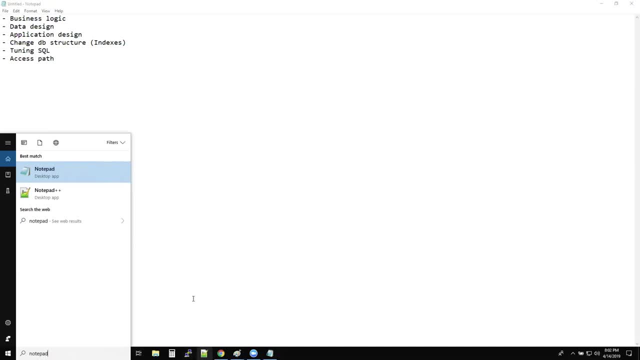 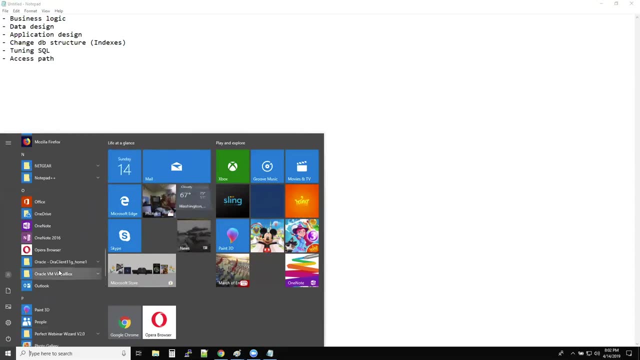 different ways to access the access path. So one of the ways I can open notepad on my system, like I can go to search notepad and hit enter right, this is one way, or I click here and then I'm not sure I need to browse through this one. I need to go. 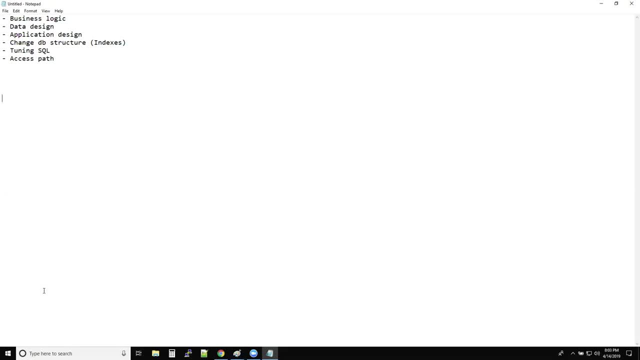 to n, m, and, and this is like notepad plus, plus, and then I don't see the notepad that I wanted. Right, This is another way, or what I can do is I go, I can go to run, I can open notepad. and I think it should open notepad right. So this is another way I can go to run. I can open notepad and I think it should open notepad right. this is another way I can go to run. I can open notepad and I think it should open notepad right. 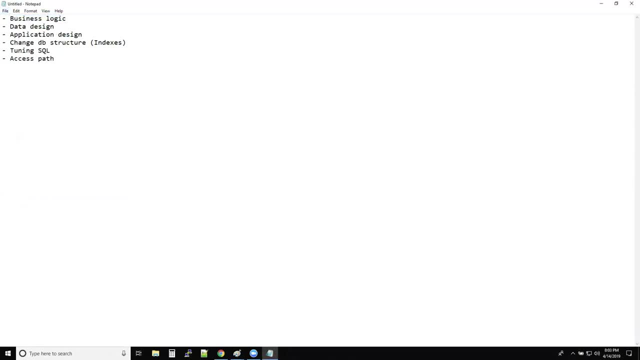 it works. or I can go to file, I can click on new, or I can right click and click on notepad. Can you see to open one notepad? there are so many ways The same thing happens in real life To go from destination A to destination B. there are. 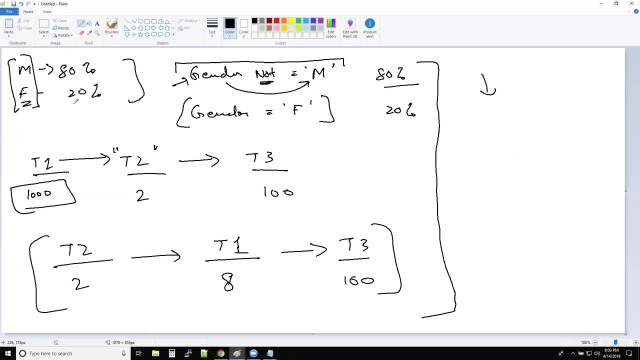 multiple ways And, like paint, I can go to file, click on new, I can press Ctrl N on my keyboard or I can right click and click on paint. Again, I can go to search type paint. there are multiple ways. But the thing is: 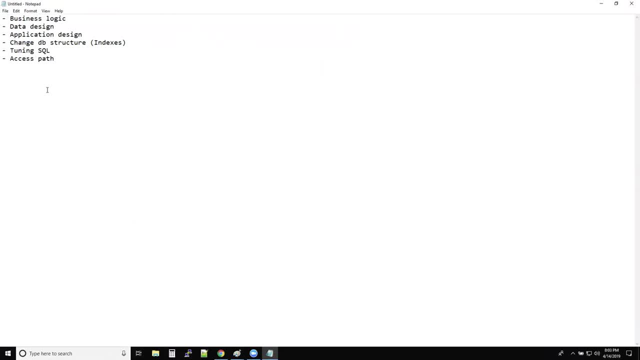 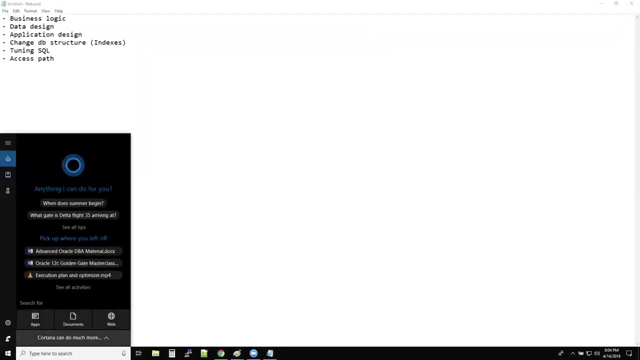 guys, you would always choose the path that costs you very less. For example, like for notepad, opening the notepad, see. let's take example one, the example one. So click. that means some resource has been involved over there, right? 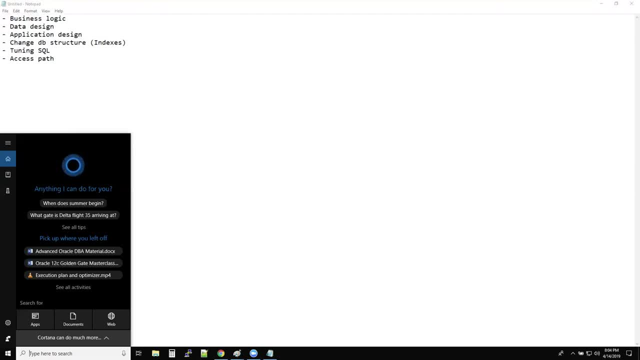 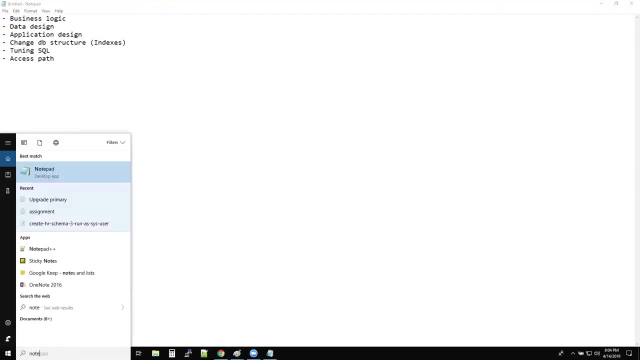 Human work was done, a click was done onto the system And then this is second level of human work, where I'm typing notepad. Okay, I just typed note and I got the notepad over there in the search result And again I'm doing human work. 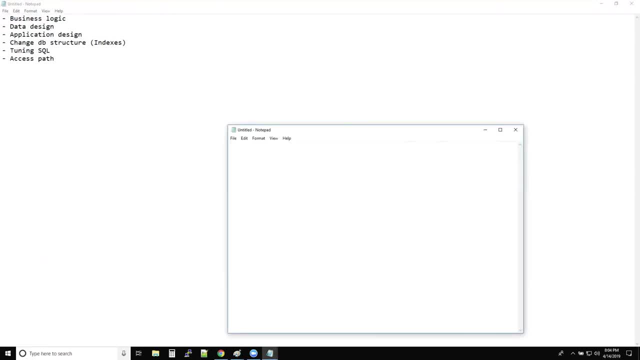 by pressing Enter. Now can you see how much effort was involved to open notepad this way? This is one, All right, And then the other one is right click And I click on notepad. Now you tell me method Was good or method two was good For me. 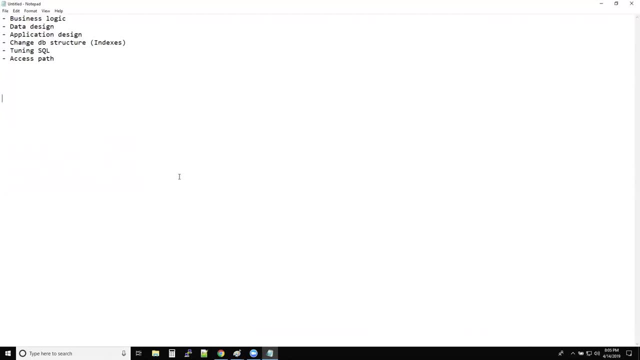 Two was good. Right Because if you go to fundamentals in the method, to the human effort involved was right click and then left click on this notepad. That means the method two is efficient in terms of opening the notepad And in terms of the amount of work that. 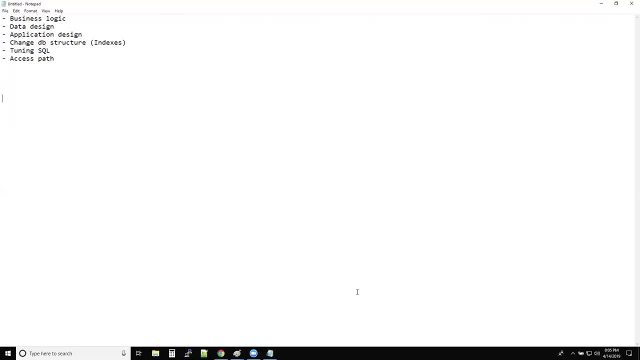 was involved to open the notepad right Gotcha, I noticed that several people graded tries out And in the two the payload of the Door認 mark. how many questions did you get from the кв12.? Oh, we only get five questions. 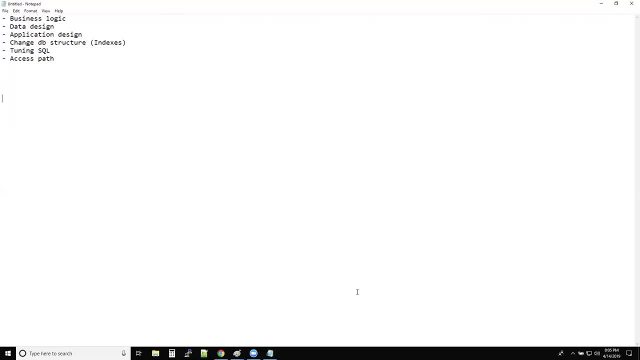 Should I actually clone that? No, but you can. I haven't seen that, Okay, Oh, wait a minute. Oh, wow, here is my något. if I click a mapped in tired, then you can't get kanji out of here. 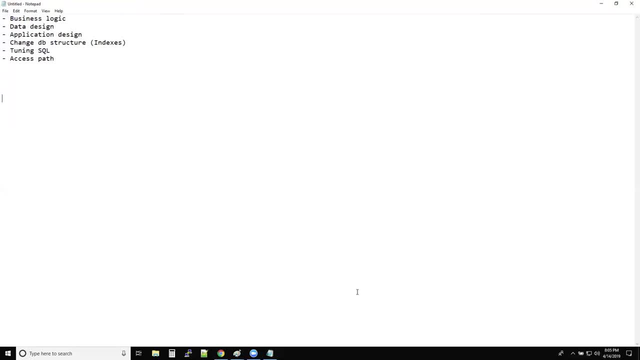 Wow, the best plan, right. so that best plan is nothing, but it consists of the cost involved to run a query. i think i'm actually going towards optimizer. but let's come back to access path. so, keeping it very simple for now, because optimizer is our next topic. access path means there are 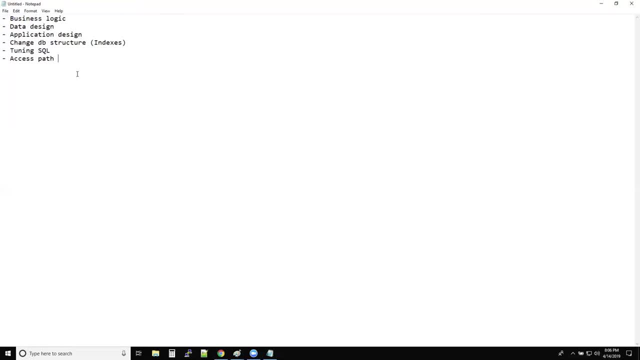 multiple ways to access the data again inside the database. it's not just one way to access the database, like, for example, should the query use index or not? should the query go for full table scan? how or should oracle rewrite your sql so that it becomes a high performing sql? even oracle has? 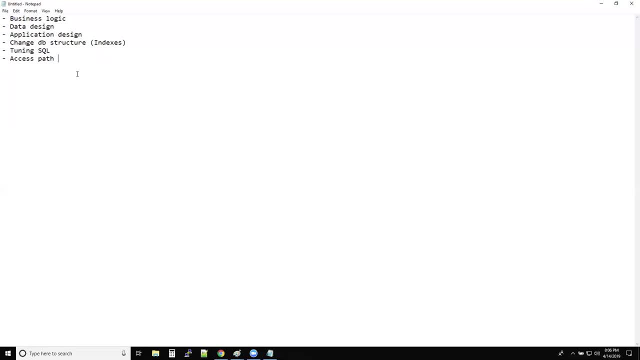 that authority. oracle optimizer can rewrite your sql query so that it becomes more effective. it might transform the sql query also. it generally happens in joins, not in a normal query, so the access path is very simple. oracle defines multiple ways to access your data and then chooses the best one. 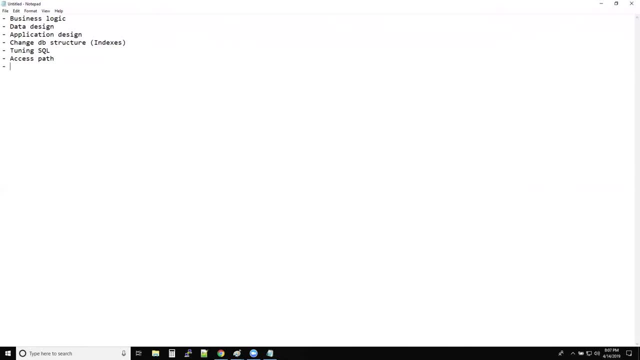 the question comes- sorry, the question that we have in terms of performance tuning: oracle sometimes might choose the wrong access path. all right, so as a dba, you need to define which is the correct access path for the sql and then try to make sure that oracle is using that particular access path. all right, so that's. 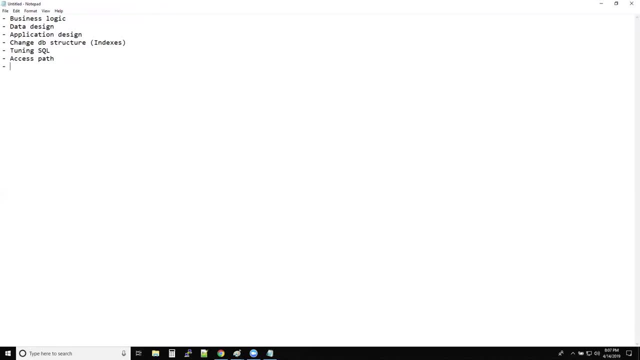 like. so what? what might be different in access path? so it's like you might create new indexes, you might remove existing indexes or you might change the type of index that is available on the table. so that way you are improving the access path. so, change to indexes. i'm making it as simple as possible. i'm not writing adding, delete or removing. 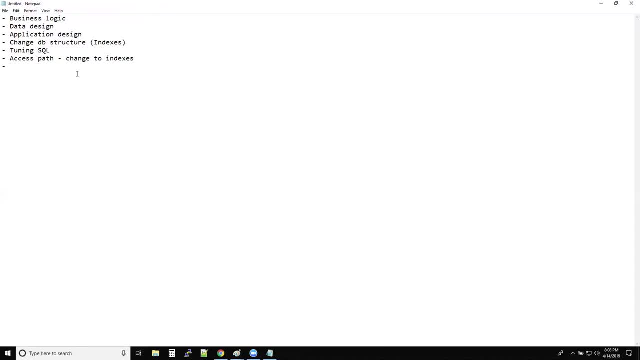 i'm just making it as change to indexes, so access path has to do with change to the indexes inside the database where it might impact how well oracle is accessing your data right. and then the next step comes in is the memory allocation, and this is also very important. 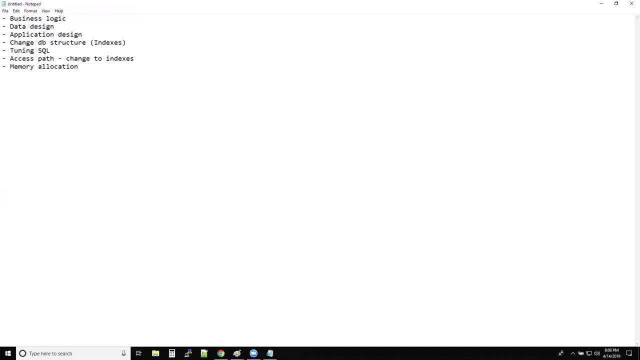 now in memory allocation. we all know instance needs good amount of memory and if there is a problem with the memory- let's take your instance- memories less, then it will always create a problem for the database to run. let's take there are a lot of sql queries that are. 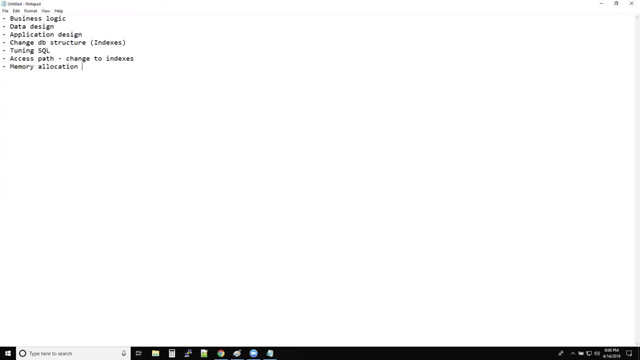 running and your instance is always going for hard parsing, then it will be a problem. and one more thing, guys: for you to be very good at sql or oracle performance tuning, you must be very good at oracle architecture. so if you don't know what is hard parsing, soft parsing and all those stuff, it will be. 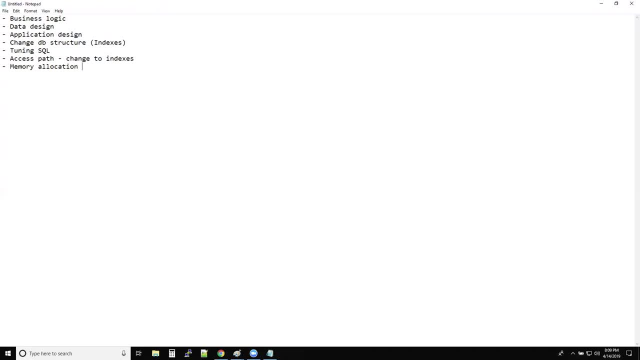 a challenge to understand all this. so in in memory allocation, mostly it is instance tuning. you tune your database instance because it resides on ram and try to understand how well uh the memory is being utilized by oracle. is it like every time, uh, 99% of your instance memory is being used, or is it like you are? 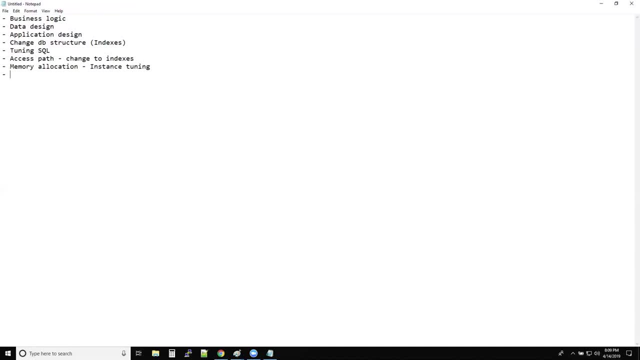 only using 1% memory that is allocated to oracle. of course, that is a good, because you always have so much memory free, but now you're wasting ram over there. like the server can use the ram for some other stuff, right? so it's it's not good to undersize your database. 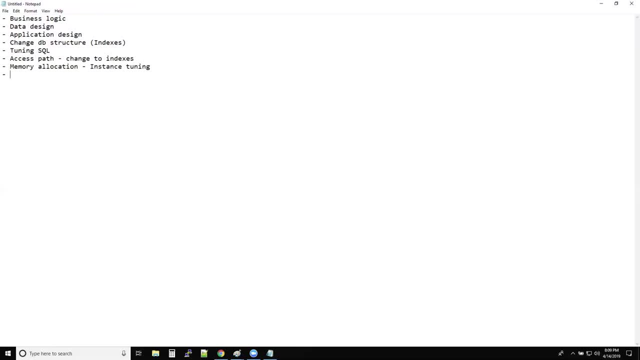 instance. it's also not good to oversize your database instance just because you have high ram. don't do it and that's. that's uh, highly stupid, like some dbas i've seen, because this happened in in my own office. a dba allocated a huge amount of ram to an instance just because 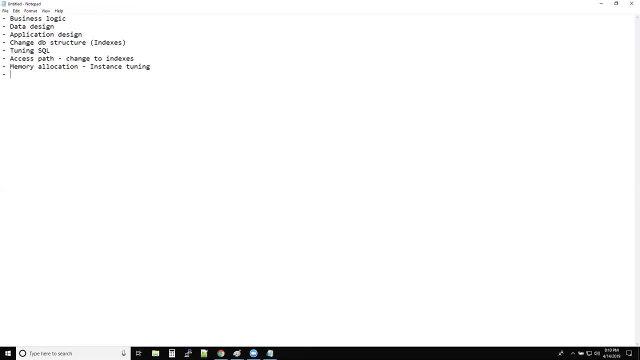 one sql was running poor, so the root cause was something else. but he thought like, okay, i'll increase the instance size so because we had a lot of ram on the server. so that's not the ideal solution. you should not go for it just like that. 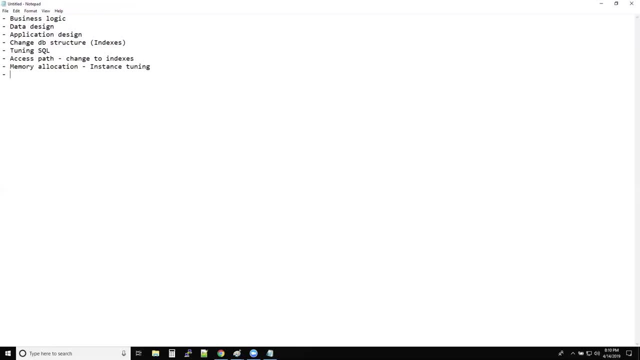 now that we have tuned the instance, we all know where does the instance reside. we know it resides on ram. do you think there might be a scenario where you have to optimize the hard disks? yes, of course. so this is where you tune the io. that's actually your physical. 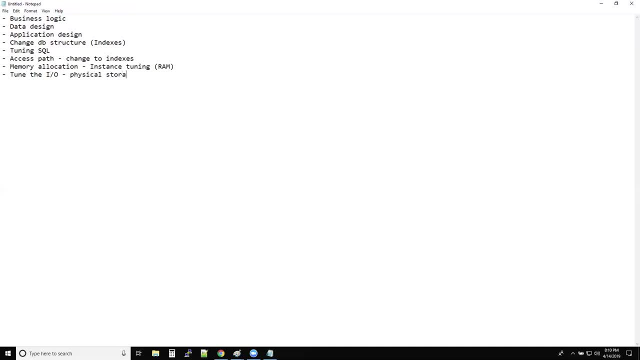 storage, physical storage. now you might have a question like: come on, arun, what can we do in physical storage? okay, this is, uh, this is something like: okay, if you are from a technical background and if you know a little bit about servers, then you might know that in general. 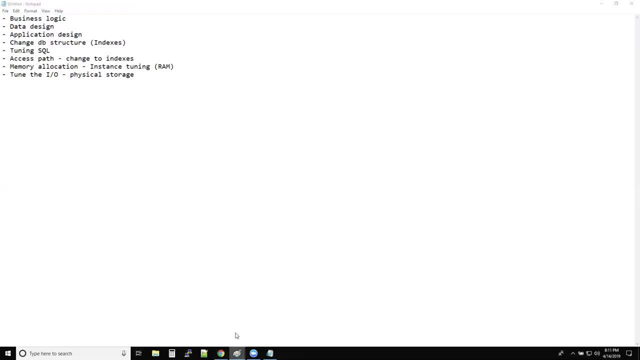 disks, guys, these are- i mean, these are the examples i'm giving from the real world scenarios that we face. all right, so, even though you might not get these problems, but that's okay. so what happens is like: let's take, you have multiple hard disks, okay, so how much time? we have ten. 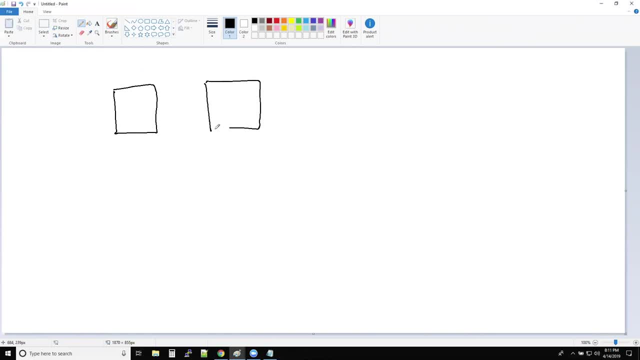 minutes more. so you have two hard disks, right, and we all know that in a hard disk there will be a cylinder and there will be a read- write header, correct? now, in this case, what happens? let's say you install your database on this one hard disk. then what will happen if the 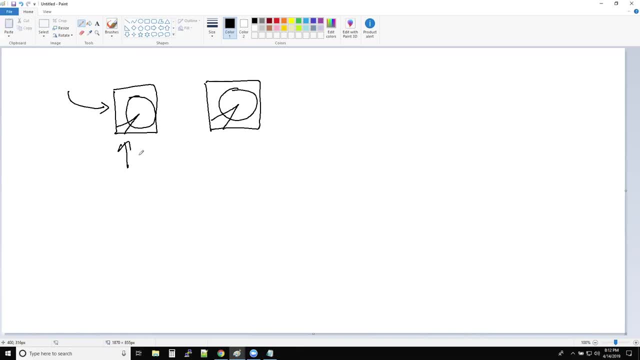 users are trying to insert into the database and in the same time users are selecting from the database. at that point of time this one hard disk structure might not work well. so can you move the data in a way that all the tables will where inserts happen? they are on hard disk two and all the tables were reporting or selects happen they. 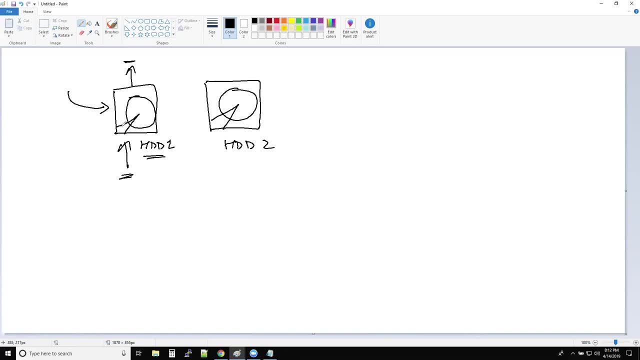 decide on hard disk one. in this way, what happens is you have to are your headers. this is: are you right? this is the i o header, so i o header one and the input output i o header two. now for the same database. you have two people working to read and write data from multiple hard disks. so you are now. 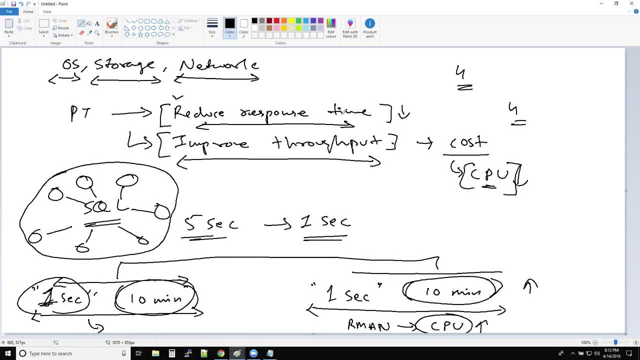 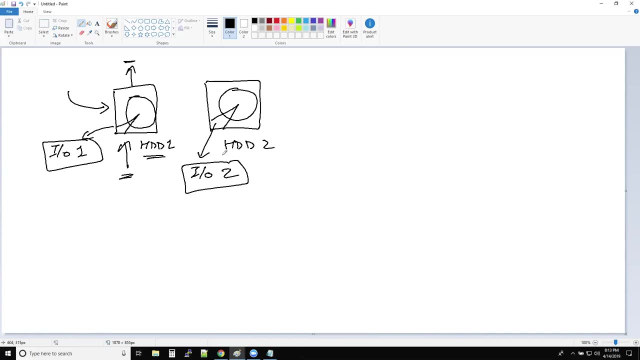 increasing the throughput. all right, if you see our tuning goal. this is also one of the important parameters. can you work somewhere on hard disk level or storage level that will improve the throughput. but my, i mean, of course. this is one good idea to distribute the data on multiple hard. 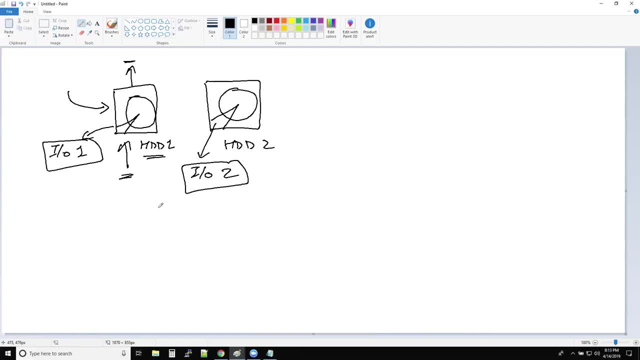 disks, and that way you get a good improvement in the data. but something from the technical side: deep inside the hard disk, every hard hard disk will have an rpm. what is rpm? rpm is rotations per minute, so in 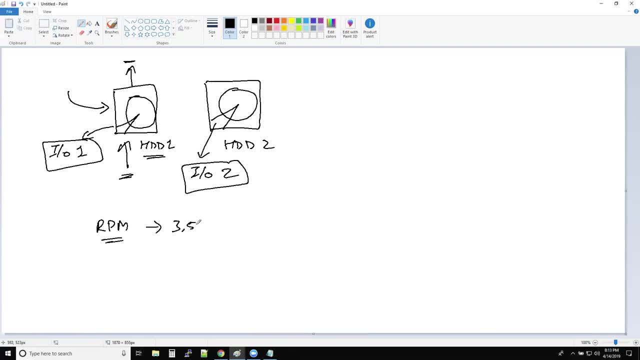 general we have hard disks which are three thousand five hundred rpm per second. that means the disk- sorry, that is rpm rotations per minute. all right, so that means this disk will rotate at a speed of three thousand five hundred rotations per minute. all right, so what happens is in. 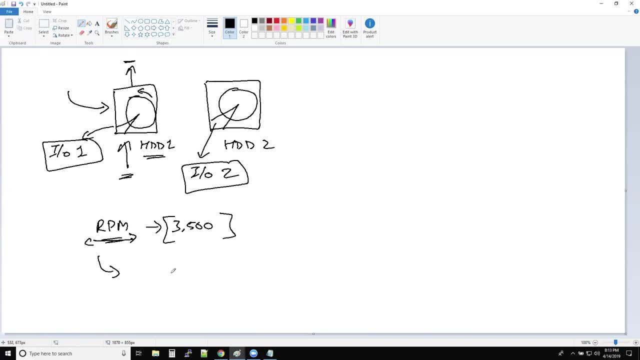 market. always there are hard disks which have improved rpm. that means there are also this, i believe, like the last one which i saw was five, sorry, seven thousand rpm. this and now, if you compare the seven thousand rpm disk is twice faster in the same one single minute. so this hard disk to this might cost you more, but the best. 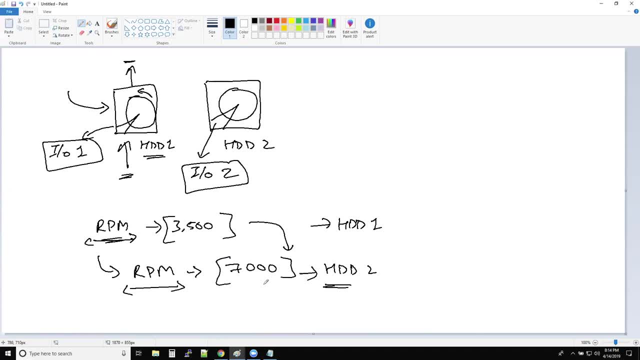 part is it rotates twice the speed of your hard disk one, so that means you can read twice the data when compared to the hard disk one. or if hard disk one takes like two minutes to read the data, hard disk two will take one minute to read the data because it is twice faster. the cylinder runs twice faster, right. 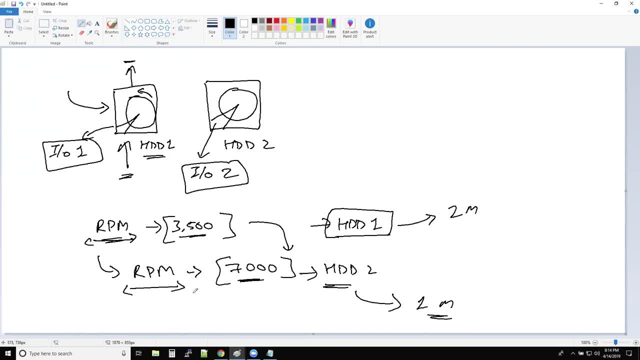 this is also a method. can you improve the storage? but, guys, very frank, storage improvement is not in the dbs hand and technically, it's not always like you have the authority to work on the storage, because storage team is completely different and, of course, depending on their performance parameters, they work on. 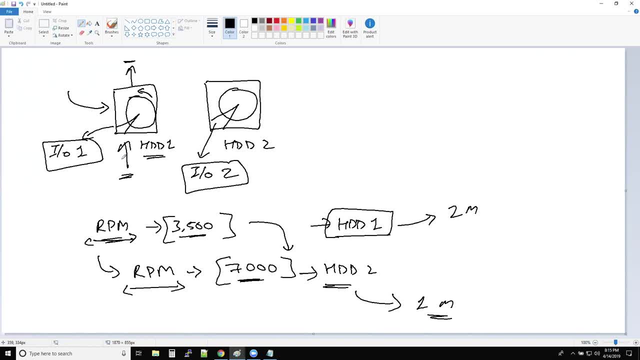 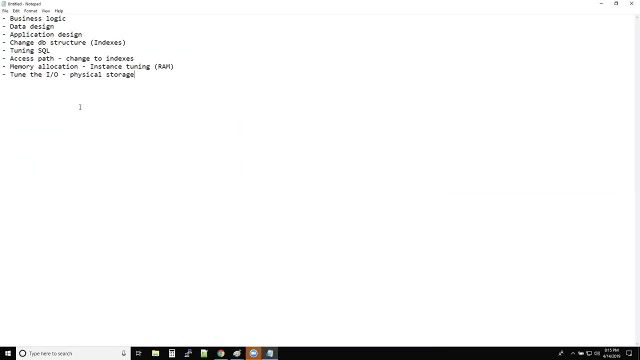 always having great hard disks, but what is in your control? in your control can you keep or distribute the data in a way that reading and writing becomes easy and much faster. that's about the tuning, the io or the physical storage, and then 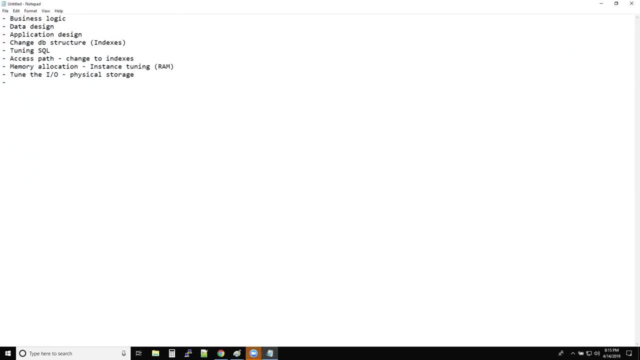 comes the. i think this should be the first one. i i don't know why i'm saying it at this stage. you, what you can do, is tuning the resources, tune resources in this one. i think it is about the avoiding the database logs, can you again? i think this can be merged back with the application design and the code, because in the resources, what you would tend to do is like: now, i think if, if we get more in details, it's like 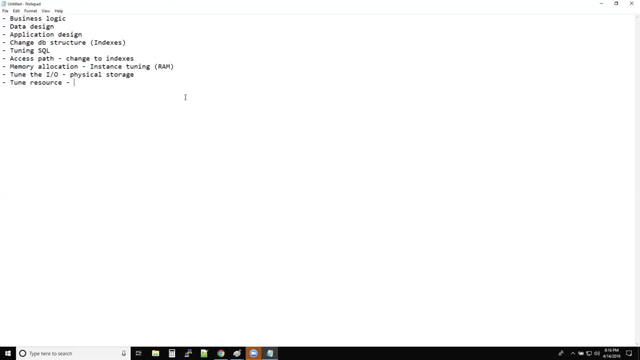 you look at what plan is being generated and how much cost that plan is happening or costing the database to run. so what you tend to do is in this step is like you work exactly inside the database to avoid the database logs or deadlocks, because those are the primary ones. i'm not getting an example that i can give you right away, so for now, let's consider locks for this. tuning resources. 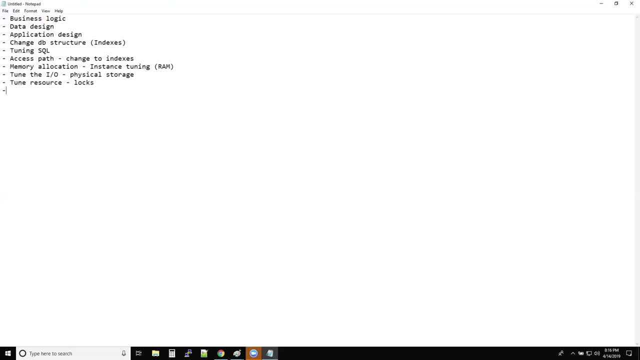 okay, all right, in the resources we also have like can. can we change the internal database parameters? because the internal database parameters? because you know we have so many internal parameters that will improve the database performance. so you might change some parameters inside database based on the application recommendation or the architecture recommendations. that will improve the entire running of the database. 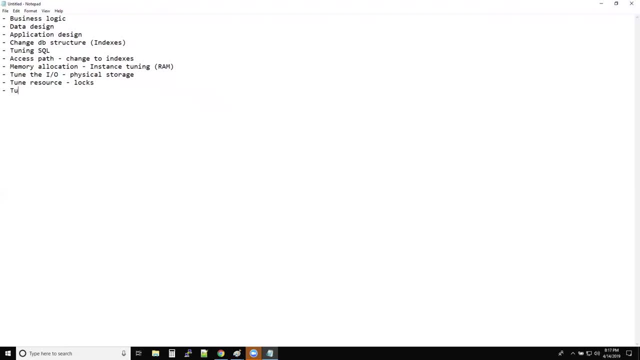 and then, finally, what you have to do is tune the server. now, this is something important, guys. as i mentioned earlier, oracle dba cannot always take the blame for a slow running query. what if there is a problem with the server? the server cpu needs to be upgraded because there is a heavy load on the cpu. then what do you do? you have to tune the server right. so, ultimately, if you see, guys, 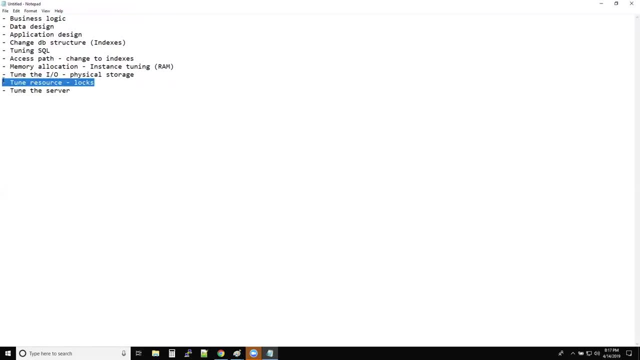 the tuning of the resources or changing database parameters, tuning of the i? o. okay, what i'll do is i'll quickly type e for external tuning. this is data design is an external tuning. then application design is an external tuning. this is the database tuning. the tuning of the sql again happens inside the database and access path, again working on the indexes, comes under the database. memory allocation is both external and the database, but mostly it has to do with the instance tuning and then this is external because it has to do with the 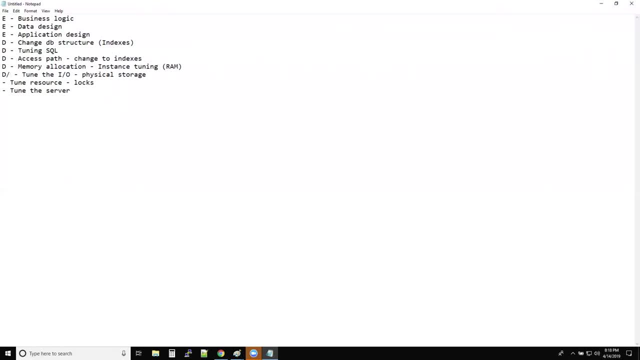 the storage team. but what i would do is i would market as e slash- sorry, e slash- d, because it is both external and database dependent. tuning of resources is database dependent and tuning of the server is external. now, if you look at the performance tuning, can you see? it is like fifty, fifty.